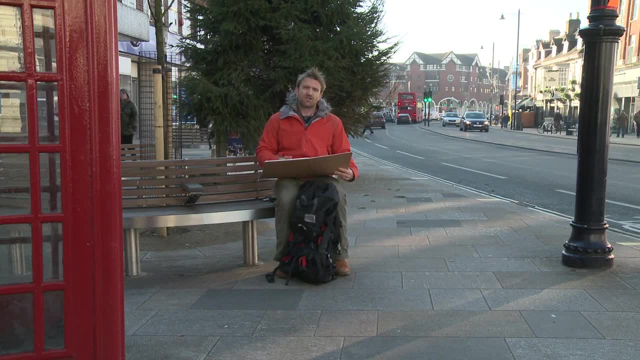 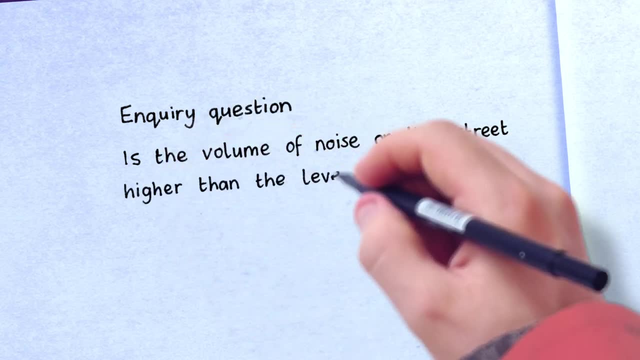 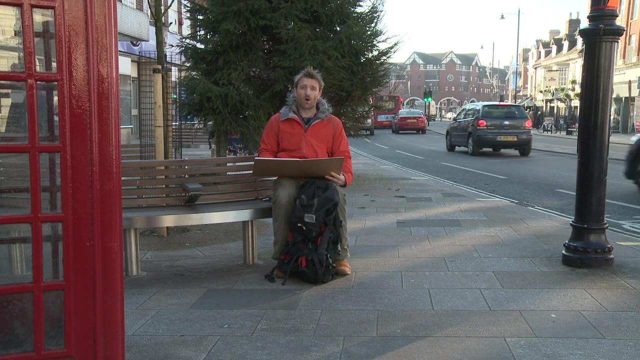 or an inquiry question you want to investigate. So it seems pretty noisy around here. So how about? is the volume of noise on this street higher than the level recommended by the World Health Organization? After an inquiry question, you need some evidence. I've downloaded an. 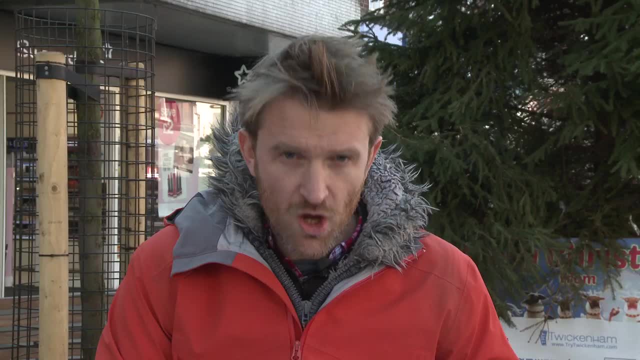 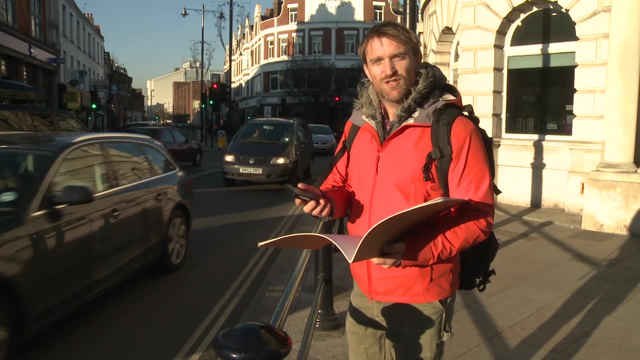 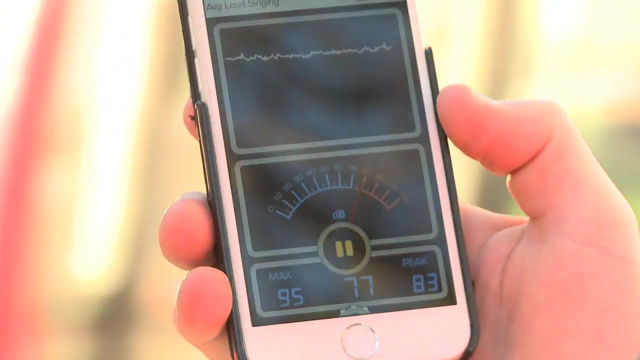 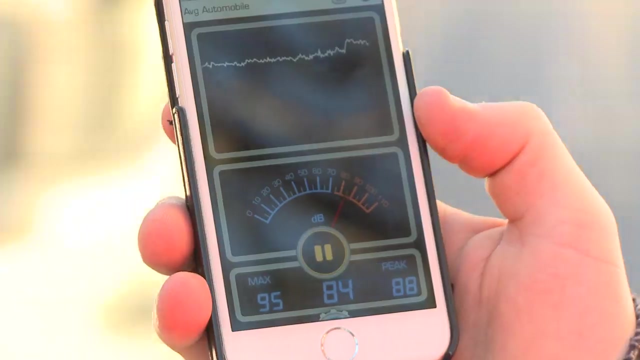 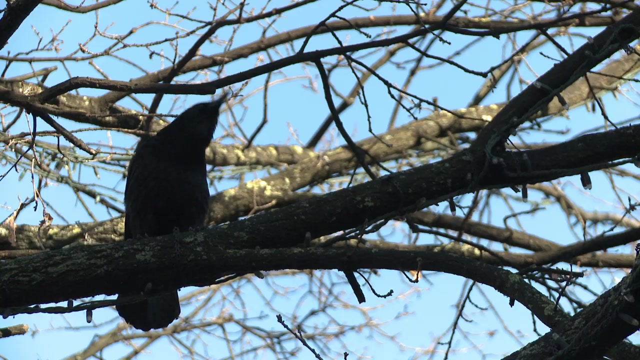 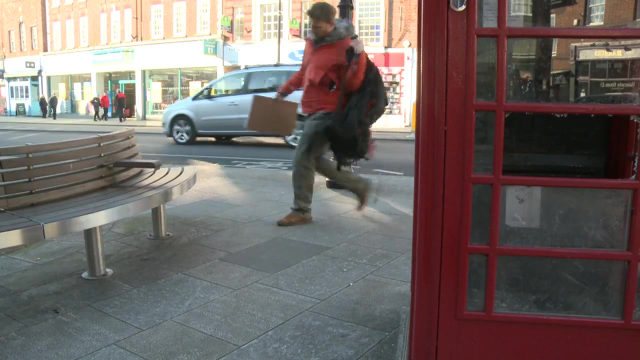 app onto my phone to measure sound levels in this area, So it's time to get some data. It's always good to do a risk assessment before you start. I'm safe behind this railing. Now let's turn all this data into something useful. This is my primary data recorded in: 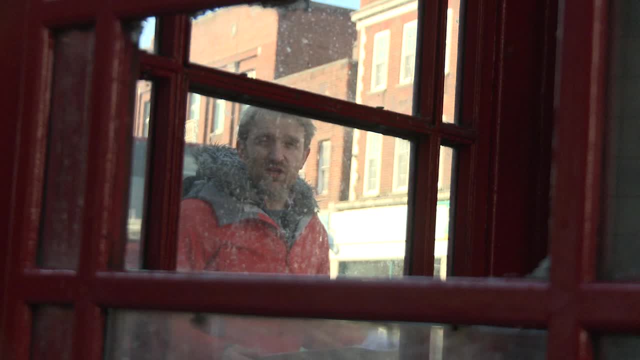 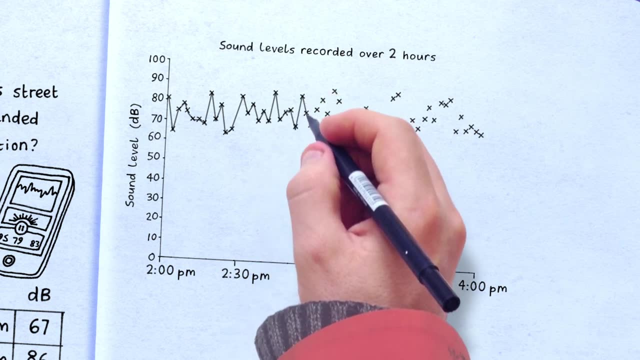 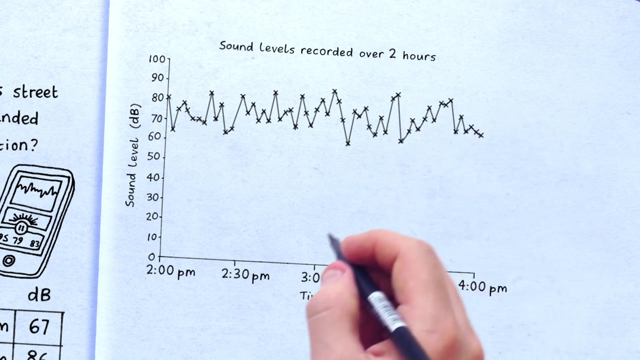 decibels over the last few hours. In fieldwork you always want to present data in a clear way, So here I've used a line graph. I'm plotting the readings on the graph with time of reading on the x-axis and sound level on the y-axis. The average decibel level outside. 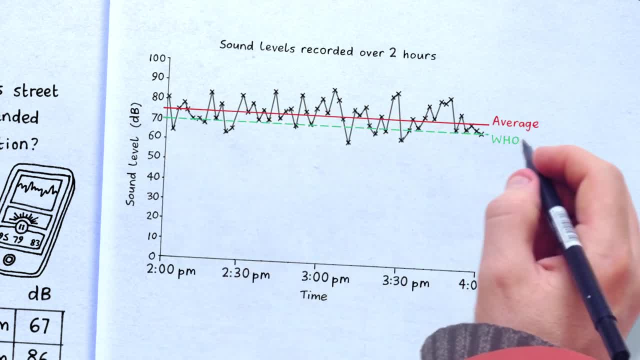 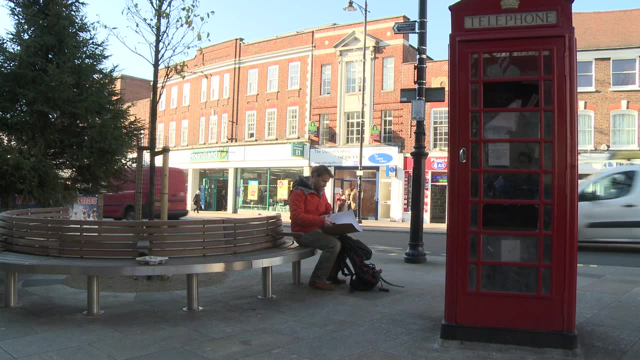 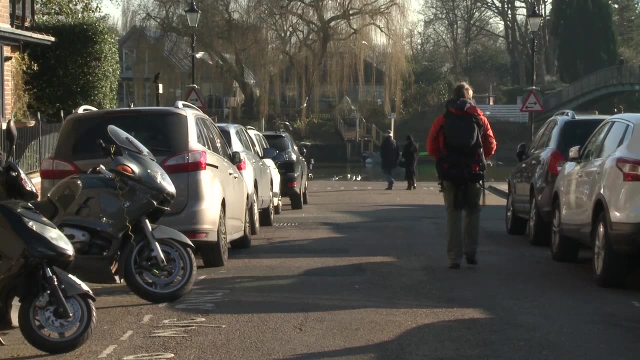 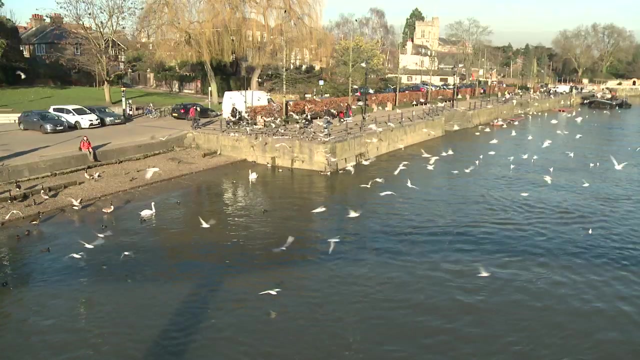 over the last few hours is 75 decibels And the World Health Organization recommends no more than 70 decibels in shopping and traffic areas. I think I'll go somewhere a bit quieter to work out the conclusion. So the answer to my- Sorry, The answer to my inquiry question, 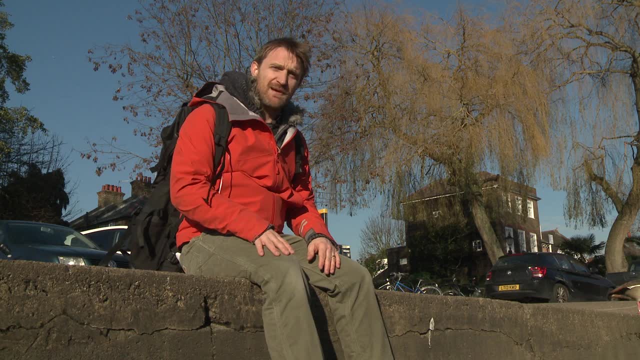 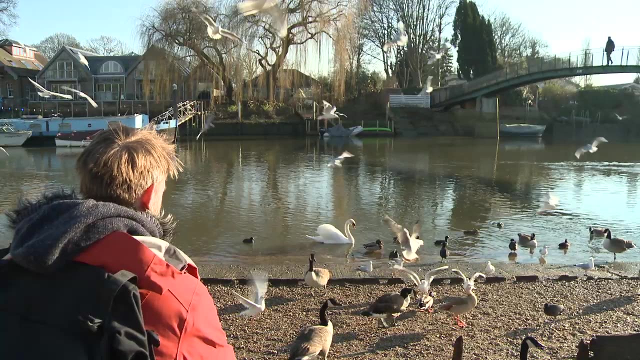 is: yes, The volume of noise is higher than recommended levels set by the World Health Organization, but not here, just 100 yards away, Every stage of fieldwork is connected. Without the right hypothesis or inquiry question, you won't develop the right method to get. 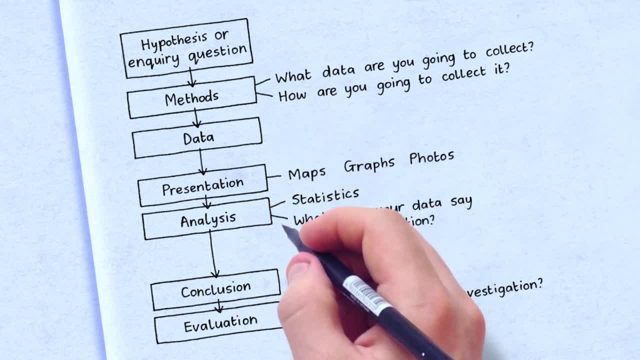 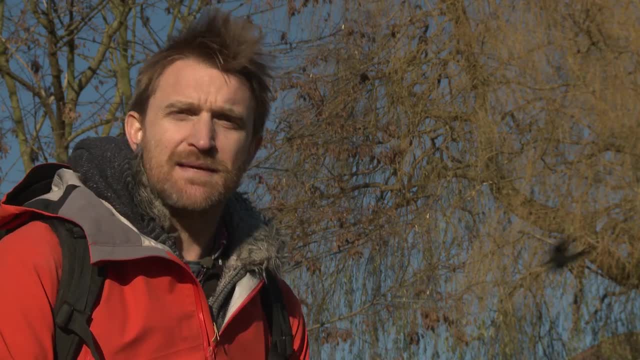 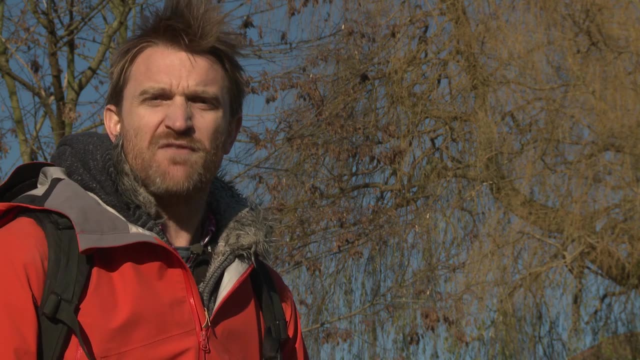 the right data. Without data, no presentation, no analysis, no conclusion And no evaluation. And my evaluation is that my data would have been more useful and actually accurate if I'd recorded it at various times in the day when the volume of traffic changed.